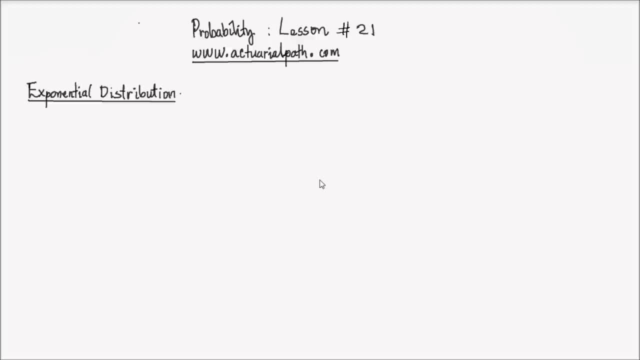 Welcome to lesson number 21 on probability from actuarial path. In this lesson we study the exponential distribution, which is used very often in different applications in engineering and insurance and so on. In engineering they typically use it to model time to failure of machines or components of a machine or computer, and so on. In actuarial science, an actuary may be interested in modeling the time to an accident or the time between consecutive accidents. 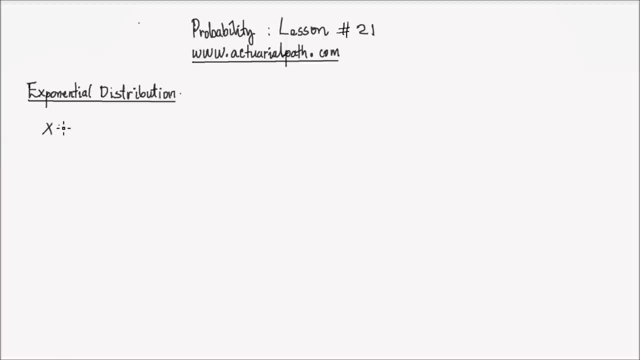 If a random variable x follows an exponential distribution with parameter lambda. exponential distribution has only one parameter, It's pdf. the probability density function of an exponential random variable is given by lambda times e to the negative lambda times x. four volumes of x greater than or equal to zero, or the pdf is zero. otherwise, 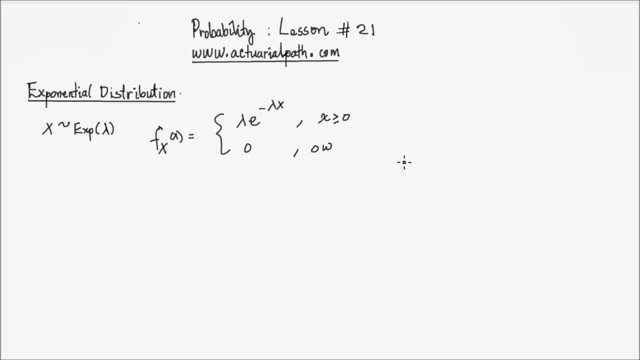 Okay And lambda is greater than zero. Definitely the support is greater than or equal to zero, because exponential distribution, as we said, is used to model time to failure. Time until something happens has got to be positive or zero. It cannot be negative. 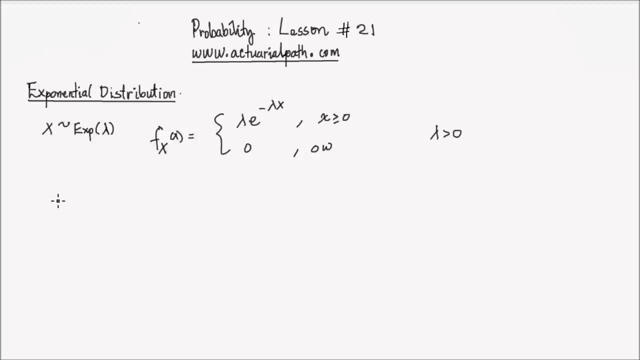 If this is a valid pdf, then we should have the integral from zero to infinity of f, dx be equal to one. Let's see if that is true. So that integral is the integral from zero to infinity of lambda times e to the negative lambda times, x, dx. 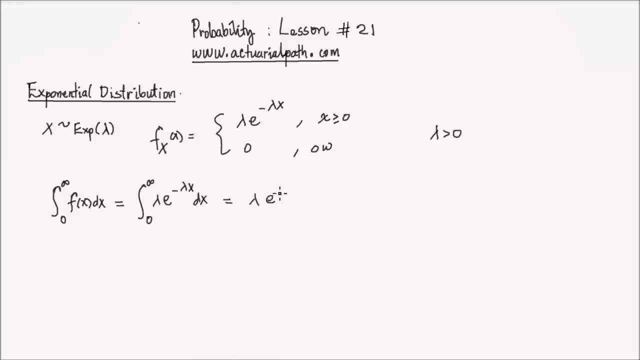 which is equal to lambda times e to the negative lambda x times minus one, over lambda limits from zero to infinity. I can rewrite this as you can cancel the lambdas, take out the negative outside and then I have e to the negative lambda. 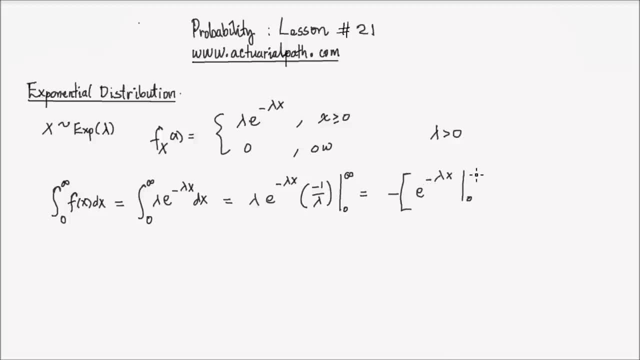 times x. lower limit, zero. upper limit, infinity. When x approaches infinity, as x goes to infinity, what you have here is e to the power of negative infinity, which is going to be equal to zero. So this is equal to zero minus. 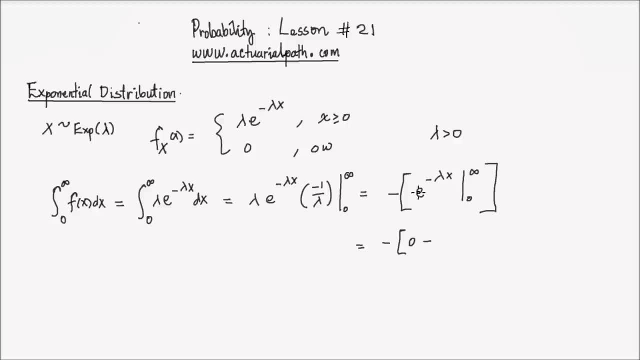 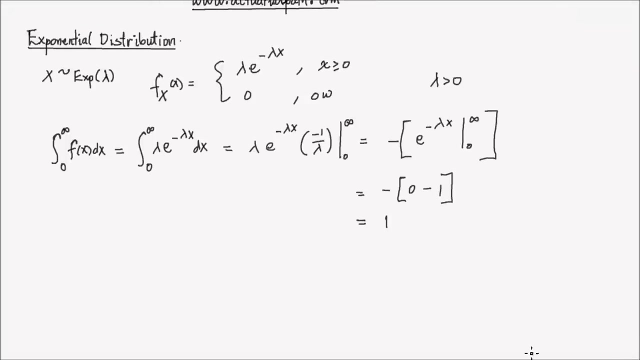 and when x approaches zero, this expression- e to the negative lambda times x- goes to one. Therefore, this is equal to one, telling us that the exponential pdf integrates to one. What I'm going to do next is find the expectation. Actually, let me do the cdf. 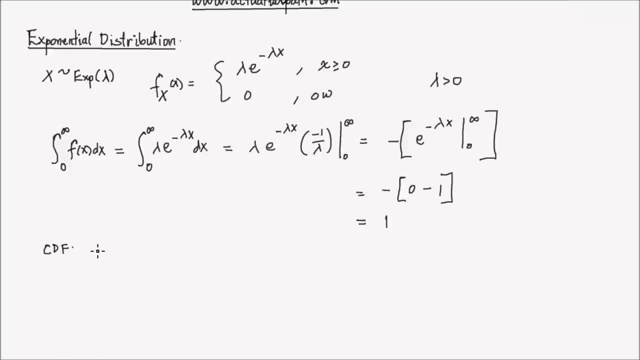 the cumulative distribution function, the cdf, of the random variable x, which is exponential with the parameter lambda. The cdf is the probability that x is less than or equal to little x. Definitely, if little x is less than zero, the cdf is equal to zero. 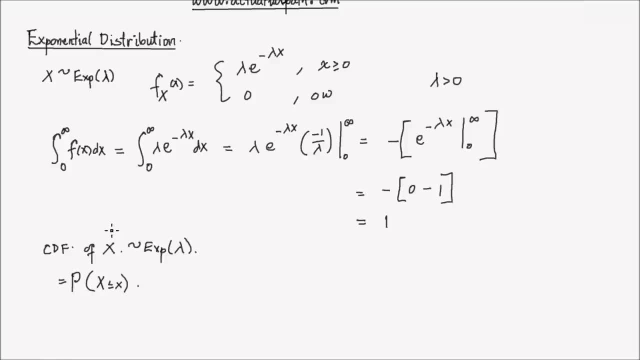 because the pdf is not valid for values of x less than zero. So this is capital F, which is the usual notation for cdfs. This is going to be equal to zero for values of x less than zero. But what is the value if x is greater than or equal to zero? 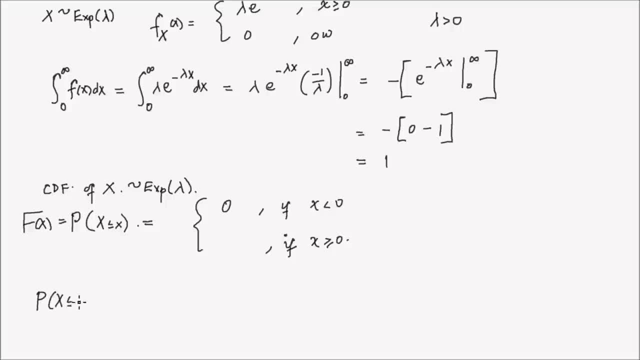 If x is greater than or equal to zero, the cdf is equal to the integral from zero to x of F, of u to u, which is equal to the integral from zero to x of lambda times e to the negative lambda times u to u. 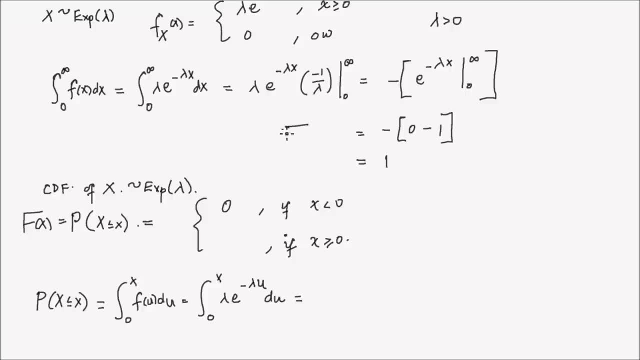 Again, very similar integration that we did here, except the limit of integration now changes from zero to infinity, to zero to x, So this is simply equal to you can do the integration. this is a very simple integration. e to the negative lambda times u. 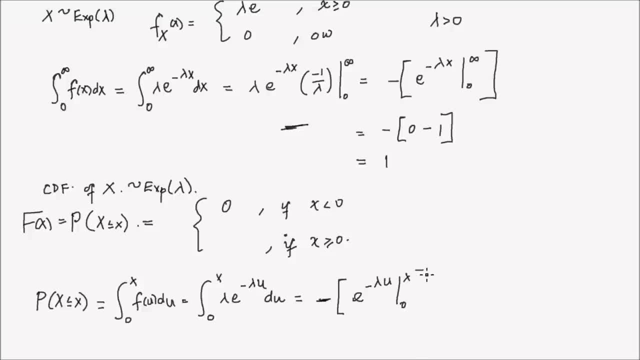 lower limit zero. upper limit: x. So when u approaches to x, this is going to be equal to e, to the negative lambda x, and when u goes to zero, this is going to be equal to one minus one. So the cdf is one minus. 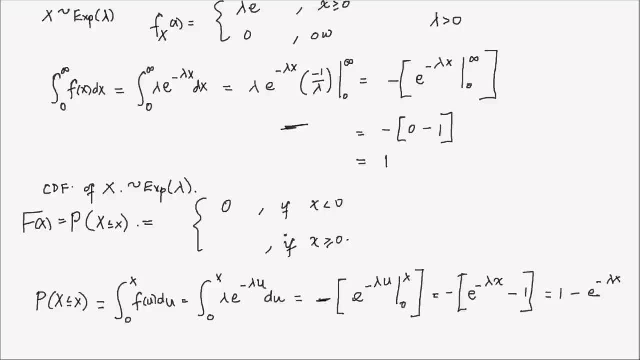 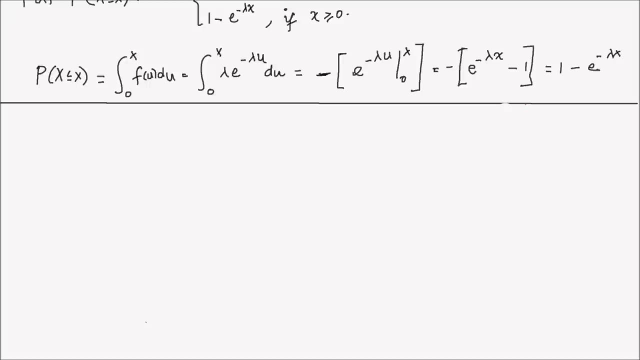 e to the negative lambda x for values of x greater than zero. So I can write this here: one minus e to the negative lambda times x. Let's find the expectation of this random variable, x. So the expectation, the expectation of x. 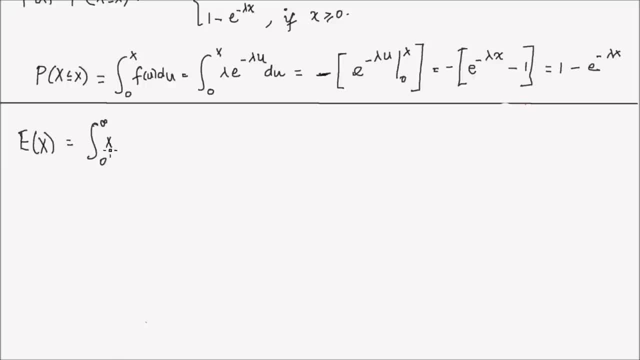 is equal to the integral zero to infinity of x times F of x dx, which is equal to the integral zero to infinity of x times lambda times e to the negative lambda x dx. We're going to apply the, we're going to apply integration by parts here. 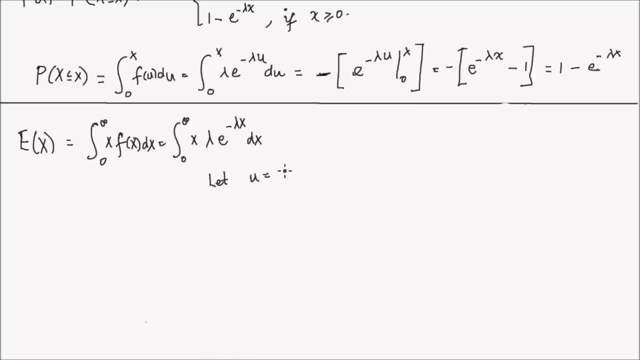 So I'm going to let u to be equal to lambda times x and dv, the differential dv to be equal to e to the negative lambda x, dx, So that that integral is simply the integral of u, dv And integration by part. 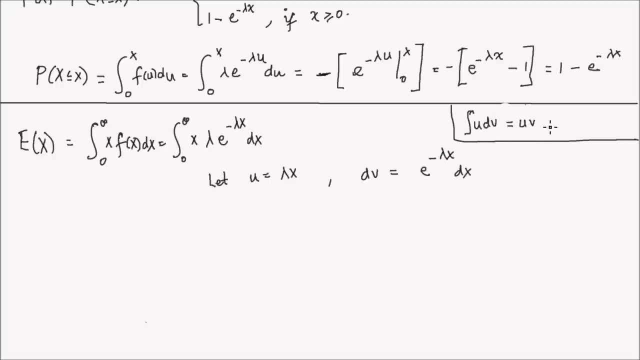 tells us that this is equal to u times v minus the integral of v, du. So we need to find du and v. But from here du is lambda times dx And v. the antiderivative of that is equal to minus one over lambda. 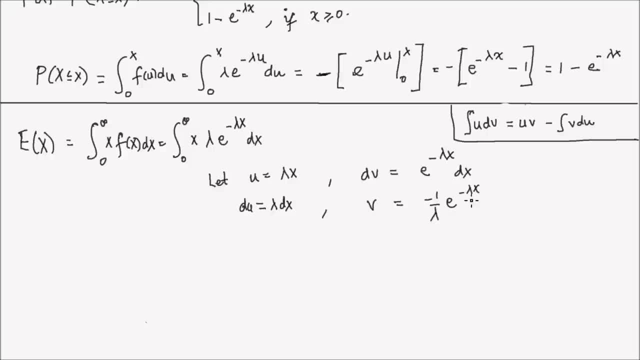 e to the negative lambda x. apply now integration by parts. We have u times v. u is equal to lambda times x times v is minus one over lambda e to the negative lambda x. So I'm going to take the negative here. 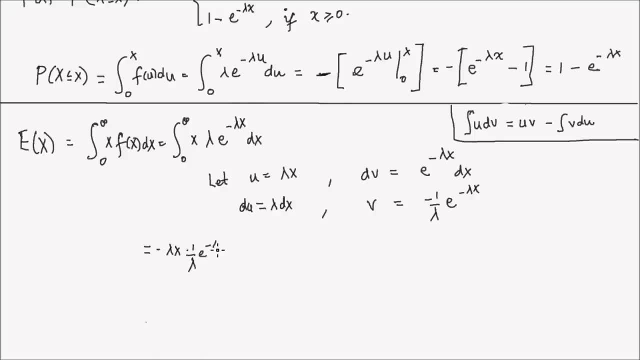 and I have one over lambda e to the negative lambda times x. Now, limits from zero to infinity, minus v integral, minus the integral of v, du, v is minus one over lambda e to the negative lambda x, du is what? 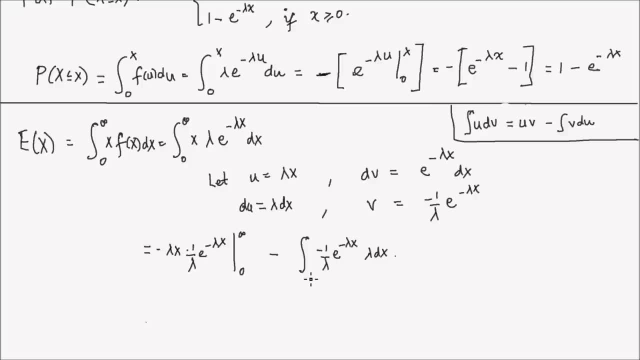 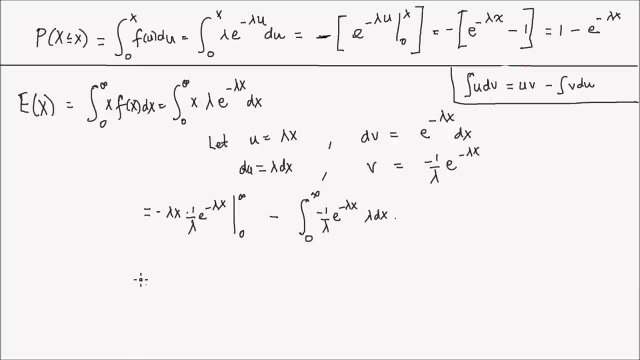 du is lambda dx. Now this is from limits, from zero to infinity. Okay, Let's cancel out things. write it in a nicer way. So this is going to be equal to minus. the lambda cancels out lambda by lambda. 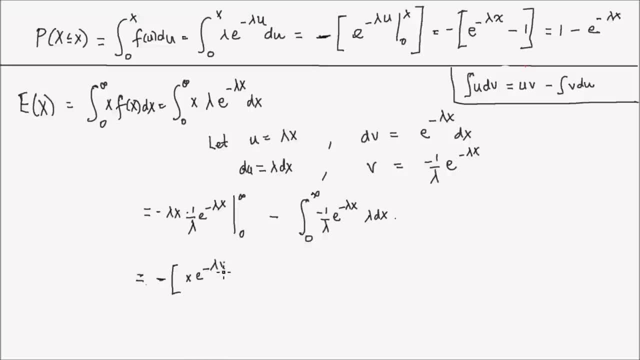 we have x times e to the negative lambda x, lower limit zero and upper limit infinity. We have minus here and minus here, so I can write a plus Integral zero to infinity, and lambda here cancels this lambda. 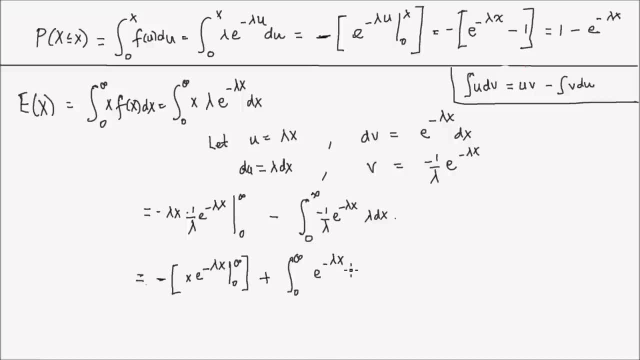 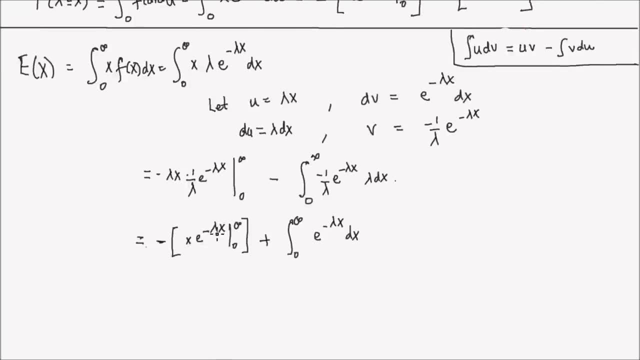 So I would only be left with e to the negative lambda x, dx. Okay, What happens to x, e to the negative lambda x when x approaches infinity? Alright, let's see that The limit as x goes to infinity. 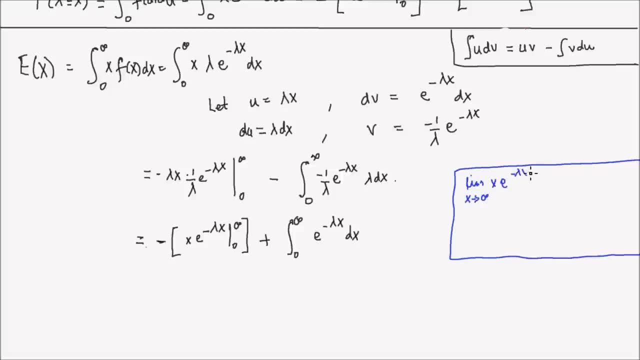 of x times e to the negative lambda x. I can rewrite this as the limit, as x goes to infinity, of x divided by e to the lambda times x. When x goes to infinity, the numerator which is x. 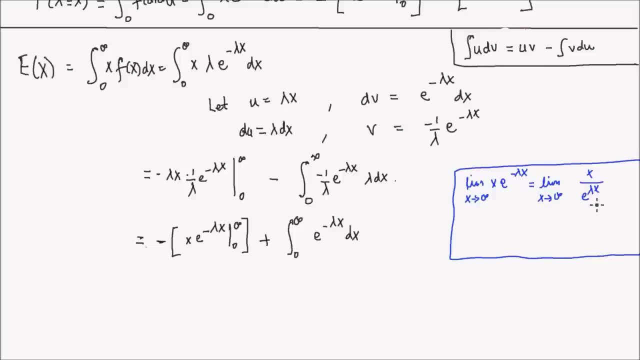 definitely goes to infinity. Also, the denominator goes to infinity: e to the negative, e to the lambda. x goes to infinity as x goes to infinity. So we have infinity divided by infinity, which is an indeterminate form. 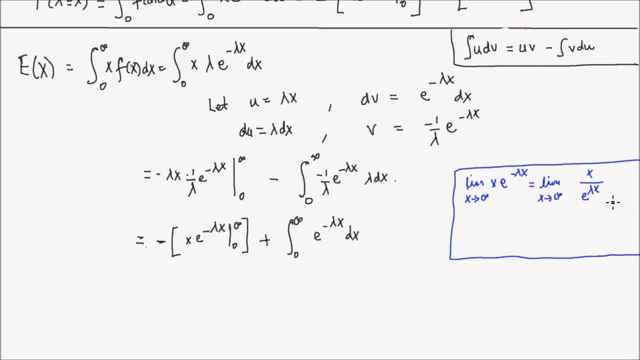 So when we have such forms, what we do is we use L'Hopital's Rule from calculus. L'Hopital's Rule is simply take the derivative, with respect to x of the numerator and also the denominator. 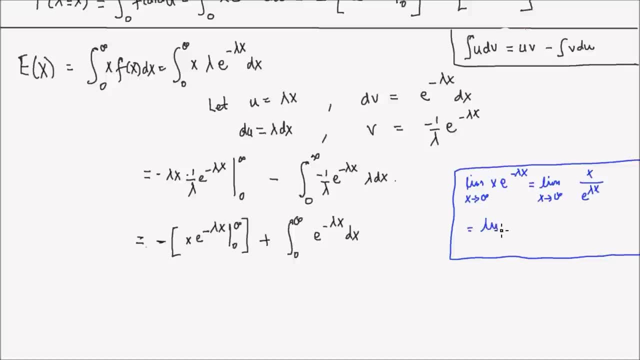 and then take the limit afterwards. So this is equal to the limit, as x goes to infinity. the derivative of the numerator with respect to x is 1, and the derivative of the denominator with respect to x. 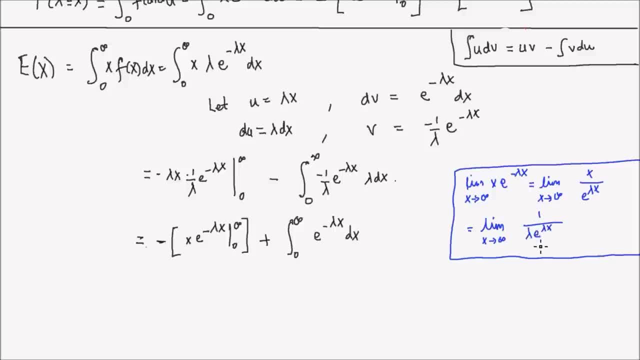 is lambda times e to the lambda x, And now we don't have an indeterminate form, We don't have infinity over infinity or something like that, So we can take the limit, a constant divided by something which goes to infinity. 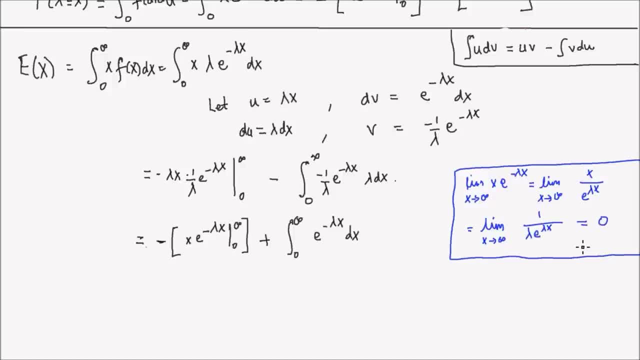 as x goes to infinity gives us a zero. So we have this equal to minus, zero, minus when x goes to zero. this is zero times e to the negative lambda, to the power of zero, Zero times any number. 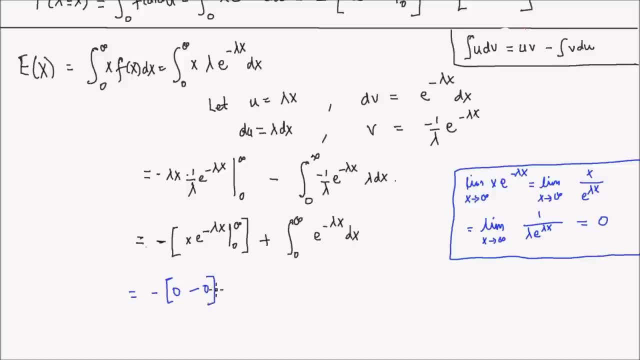 is going to be zero. So this is zero minus zero, which is zero. So this term actually entirely goes to zero. So we are left with only the second integral term, which is integral zero. to infinity of e, to the negative lambda. 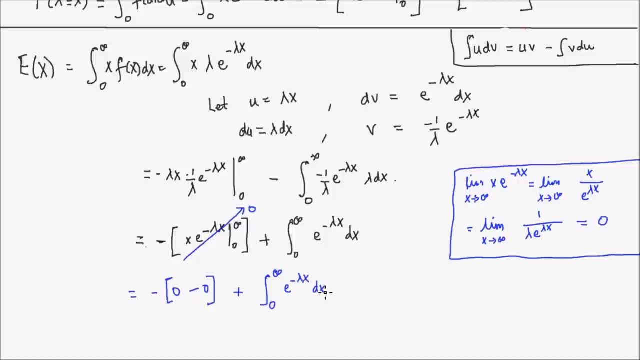 times x, dx. You can read the integral. this is a very simple integration, but there's a simpler way of doing this, which is multiply this by lambda and also divide it by lambda, so nothing changes, And you see that. 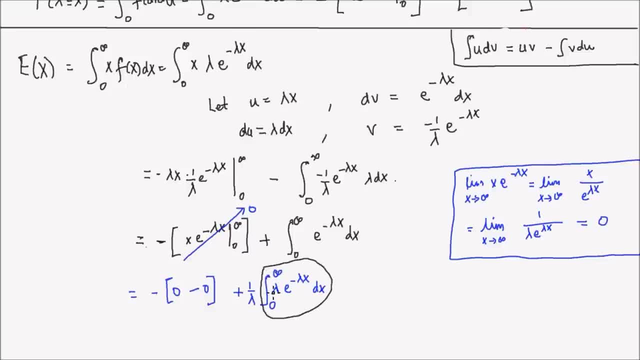 that expression is the integral of an exponential PDF. This is what you should be very good at in probability: Recognize that this is a PDF of an exponential distribution, so therefore it must integrate to one. Okay. 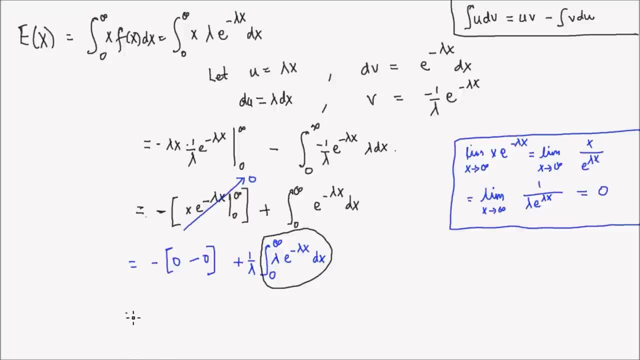 So that goes to one. What I have in circle here in black goes to one. so I have zero plus one over lambda times one which is one over lambda. So the expectation of the exponential random variable x. 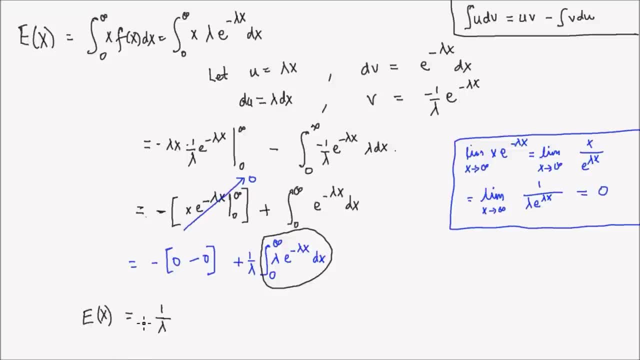 is equal to one over lambda. I think this is a very tedious way of doing the expectation. We have a nicer way of finding the expectation, which is what I'm gonna do next. That involves using the moment, generating function. 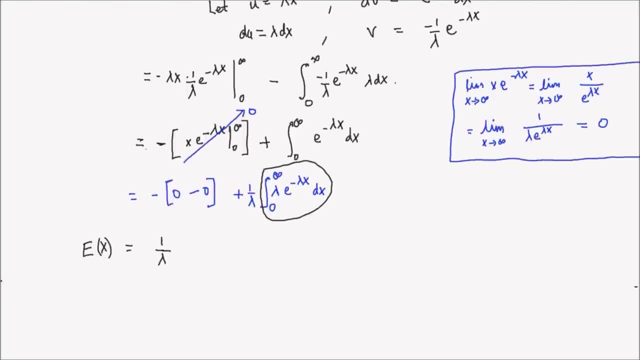 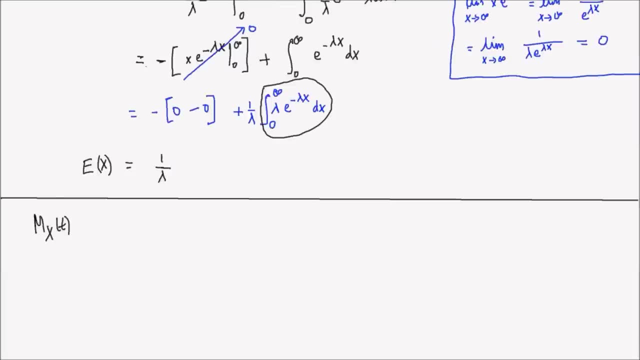 of an exponential random variable. Let's find the MGF. The MGF is equal to m. x of t is equal to the expected value of e, to the power of t times x, which, in this case, 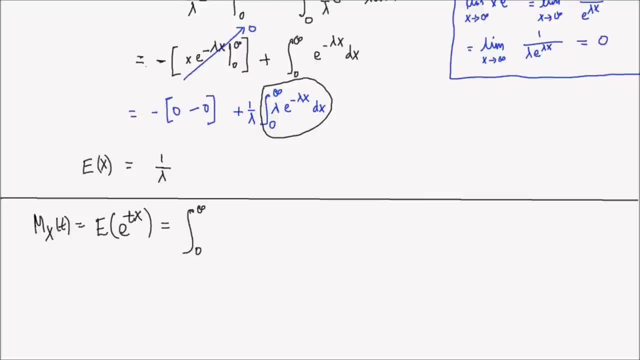 is equal to the integral from zero to infinity of e to the t x times the pdf lambda e to the negative lambda x, dx, Which I can rewrite as integral zero to infinity of lambda. 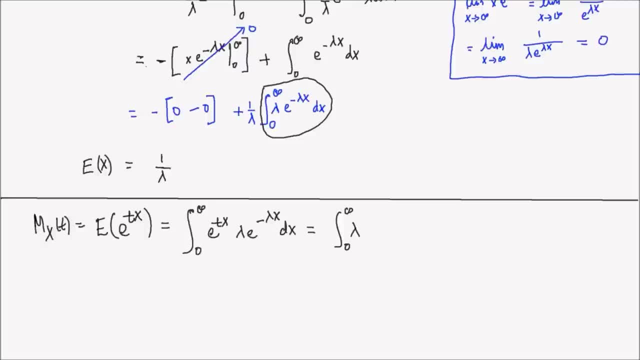 combine the powers here. e to the: what do I have? I have minus lambda x plus t x, dx, Which you could combine with. e to the: what do I have? I have minus lambda x plus t x. 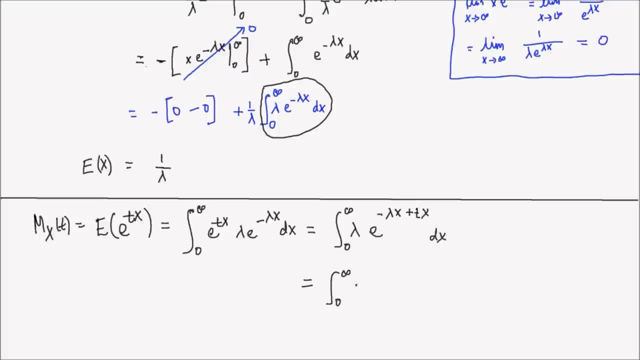 dx, Which you could combine again, simplify as lambda e to the power of minus lambda minus t times x, dx. Take out this lambda outside of the integral so you have lambda times the integral. 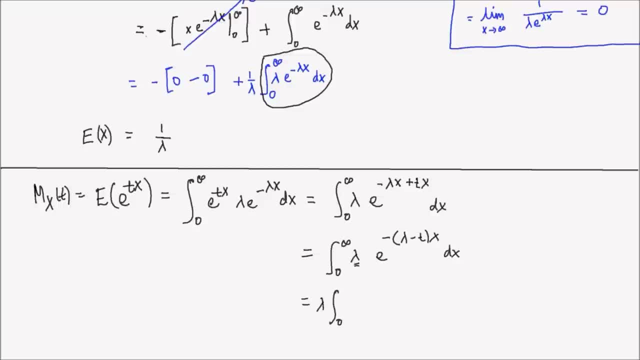 zero to infinity of e to the power of negative lambda minus t times x, dx. Now you recognize that. e to the power of negative lambda minus t- Now you recognize this looks like. 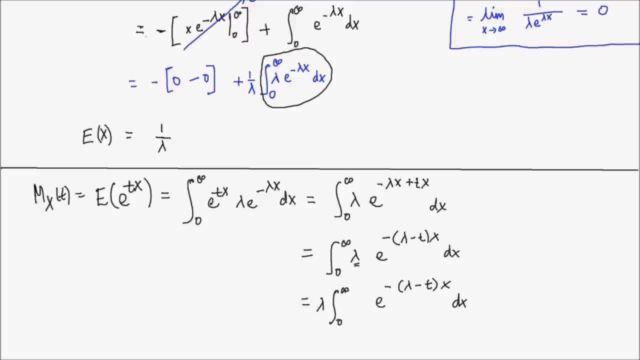 the pdf of an exponential distribution with parameter lambda minus t. So if I multiply this by lambda minus t, then this integral should be equal to one, Because I am integrating an exponential pdf. 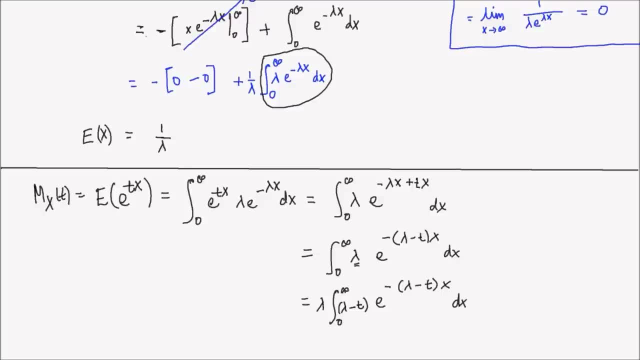 You need to be good at this. That's one of the major tricks in probability distribution, uh, distribution theory, Um. but since I multiplied this by lambda minus t, I need to divide it. 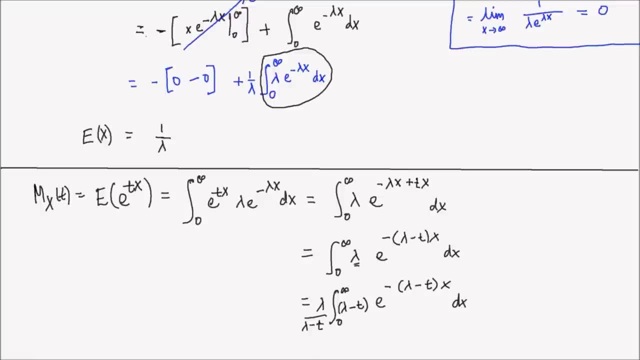 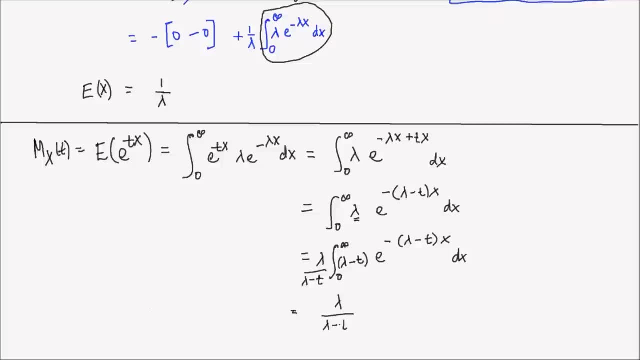 by lambda minus t, so that nothing changes. Okay, So the quantity doesn't change. So this is equal to lambda divided by lambda minus t multiplied by one. So once you have the MGF, 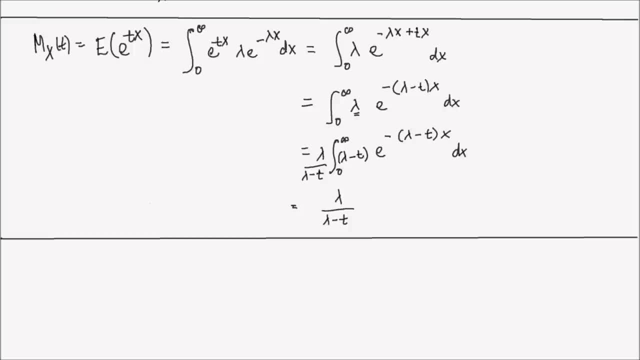 um, it's a matter of doing derivatives to find the expected value and the variance and so on. So the expected value of x is now much easier to find because you just need to find the derivative with respect to. 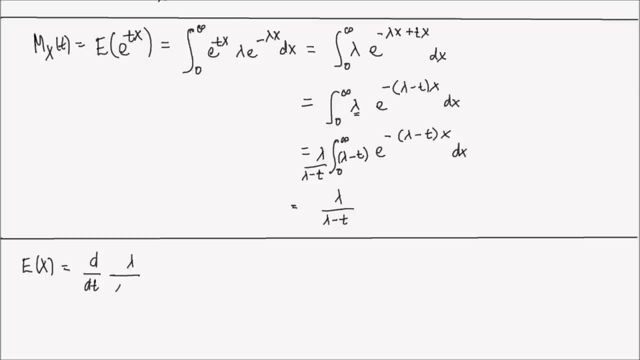 t of lambda minus lambda minus t, which is the MGF, and evaluate that at: t equals zero, The derivative of the MGF. evaluated at uh, the value of t equals zero. So 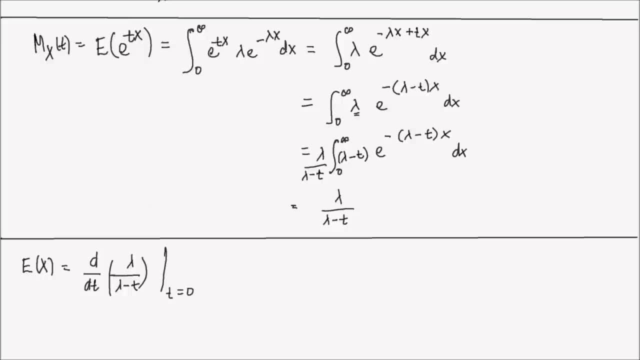 this is much easier to um deal with than doing um integration by parts. That's just my opinion, But there's so many different ways of doing the same thing. It doesn't mean one is wrong. It means that 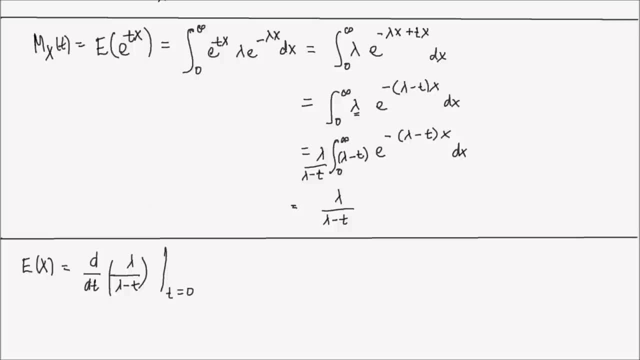 some are easier than the others. So uh for you, you could uh when you solve problems, especially in exam settings. you want to find the quickest way possible to do a problem and you don't waste your time. 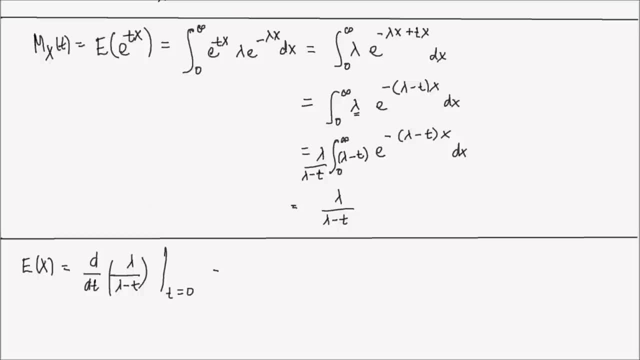 Okay, So let's find this derivative, and that derivative is equal to lambda, actually negative lambda times lambda minus t square. But then I have to take the derivative of uh, lambda minus. 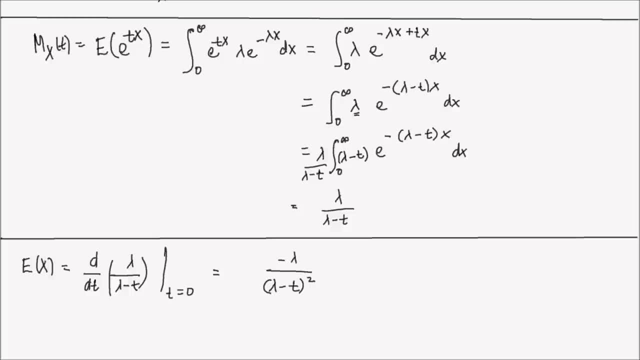 t by chain rule uh, and the derivative of lambda minus t with respect to t is negative one. So multiplying by to get rid of the minus and evaluate this at t equals zero. 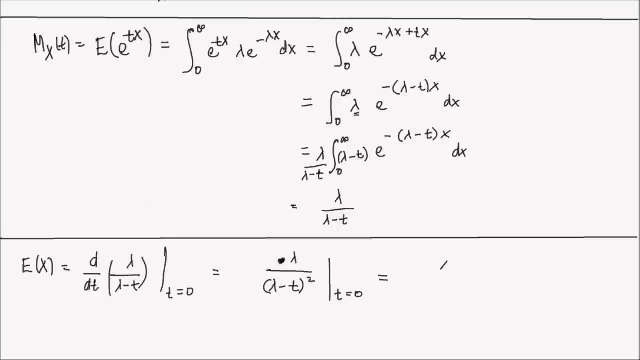 and that is equal to lambda divided by, that looks like an x. oh, lambda divided by lambda minus zero square, which is lambda square, that gives you one over lambda. So we found. 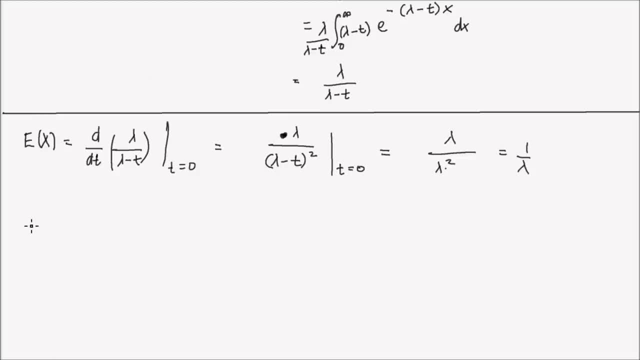 the expectation using the MGF technique, which I think is much simpler to do. Likewise, when you find the expected value of x squared, you can use the formula the integral zero to infinity of x squared. 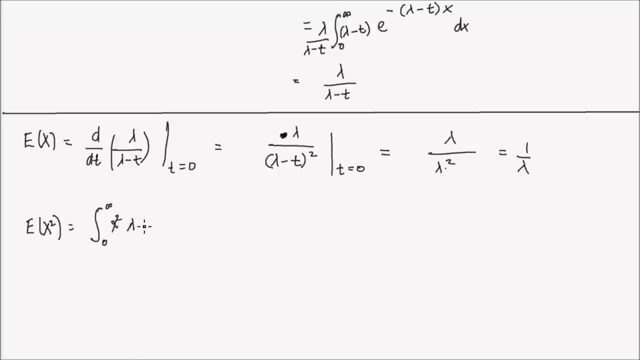 f of x dx, which is lambda e, to the negative lambda x dx. If you follow this route, you're gonna have to use integration by parts twice to solve this integral, which is fine, it's not a problem. 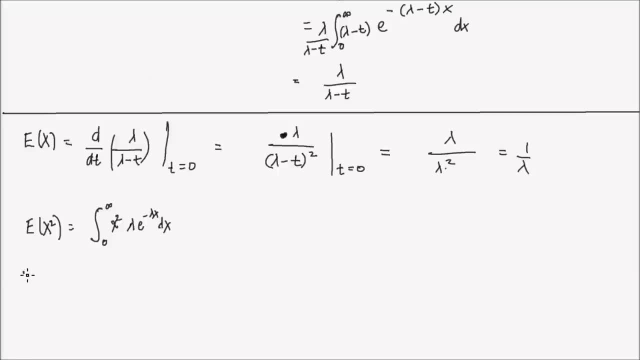 but it's much quicker to use the MGF technique. If you do that. the expected value of x squared is the second derivative, so d squared, dt squared of the moment generating function evaluated at. 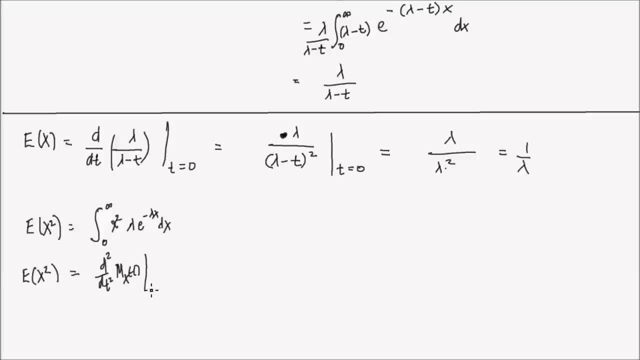 t equals zero. Now, this is the first derivative of the MGF. So to find the second derivative, you simply take the derivative of the first derivative of lambda divided by lambda minus. 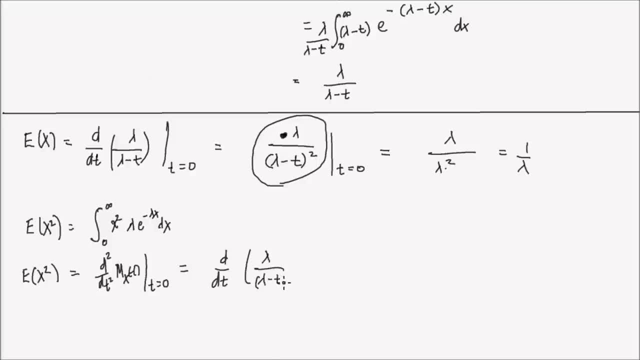 t. So minus t squared, And then evaluate that at t equals zero, And that gives you minus two lambda divided by lambda. minus t to the power of three. Now, 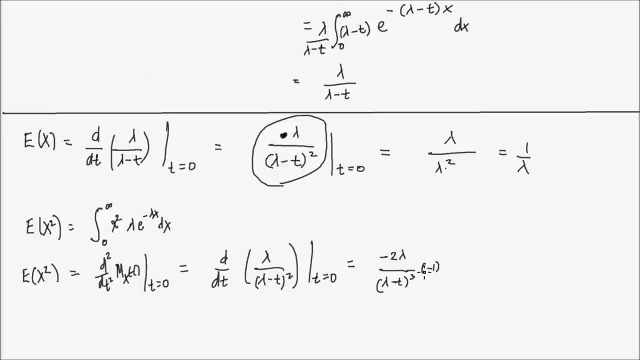 times the derivative of lambda minus t with respect to t, which is negative one, And evaluate that at: t equals zero. So when you plug in t equals zero, you get. 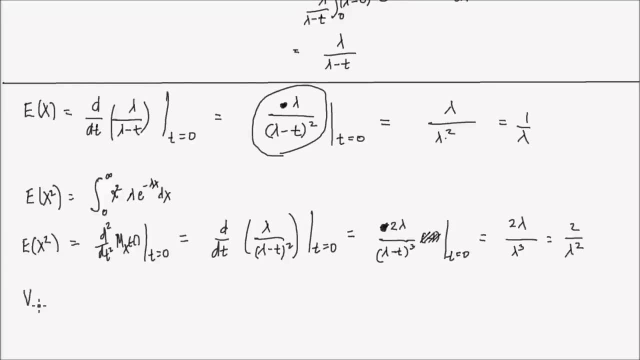 two lambda divided by lambda to the power of three, which is two over lambda squared, And therefore the variance is the second moment, which is two divided by minus one. 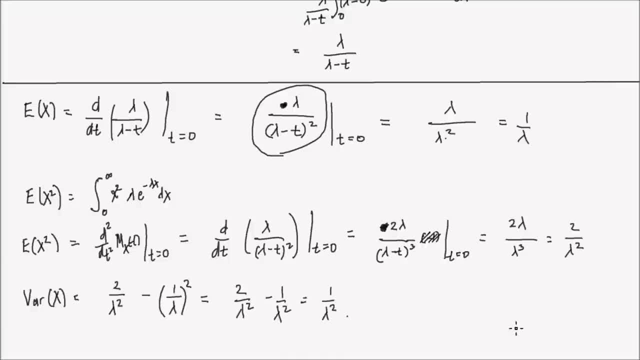 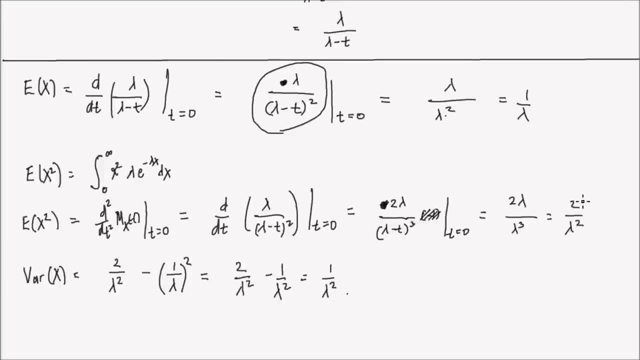 over lambda squared, which is one over lambda squared. So for an exponential distribution with parameter, with the rate parameter lambda, the expected value is one over lambda And the variance 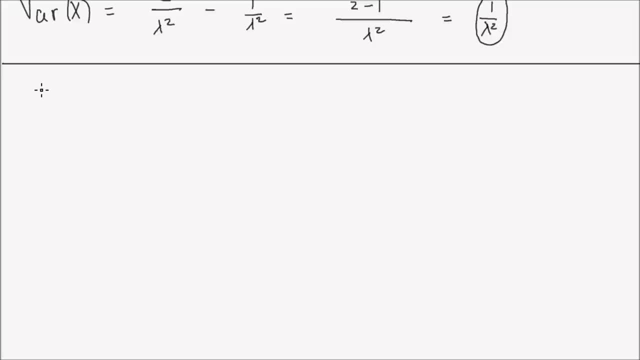 is one over lambda squared, So the variance is one over lambda squared times two plus one over lambda squared, So we have the value of x. 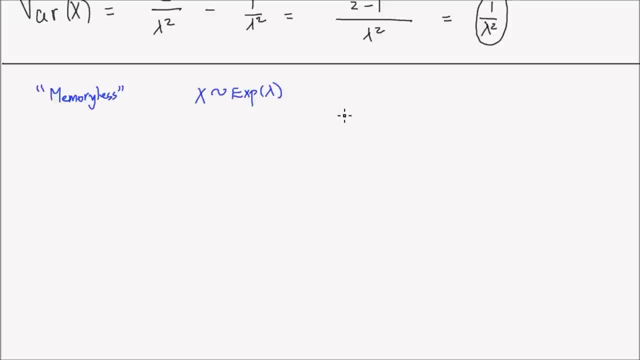 x squared over lambda squared And the variance is one over lambda squared. Since lifetime distributions are typically non-negative, I'm going to draw a number line starting from zero. Okay, say that's point zero. 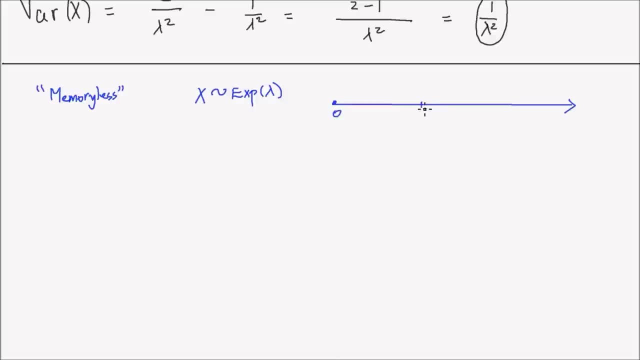 Suppose this time this point is point s, so this length from zero to s is s units of time. And let's say this point here is s plus t, So this interval from this point to that point has a length of t units of time. 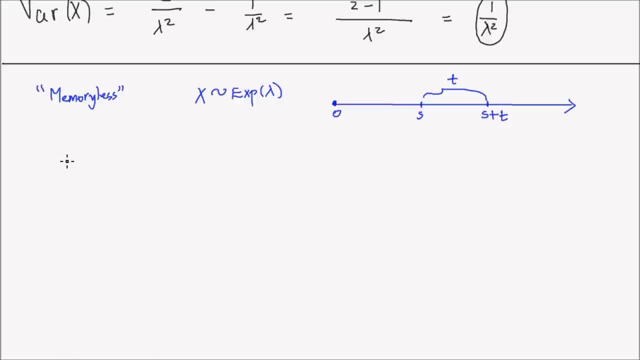 The question I want to ask is: what is the probability that this equipment will be functioning or will be functional after time t plus s? That is, the probability that s is s, Given that x is greater than s plus t, Given that it was functional, or given that it is functional after time s. 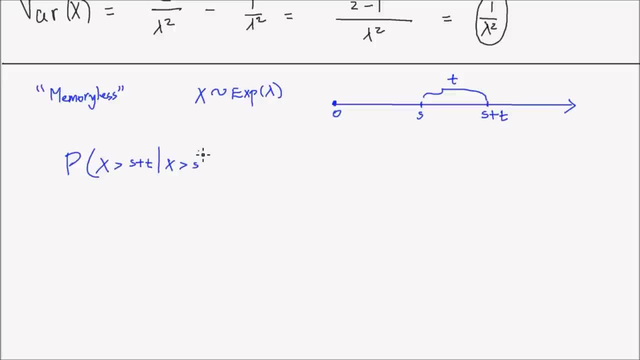 Given that x is greater than s. Another way to express this is: if I tell you that this machine has been working or has been operational until time s, what is the probability that it will be operational for at least additional time s? What is the probability that it will be operational for at least additional time s? 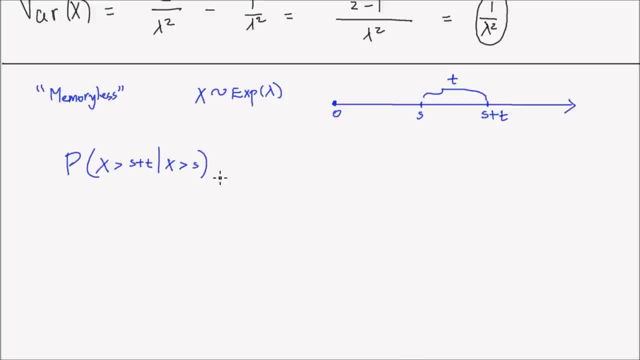 What is the probability that it will be operational for at least additional time s? So that is what this probability is asking. So that is what this probability is asking, And memoryless property says this: It doesn't matter how long this equipment has been operational. 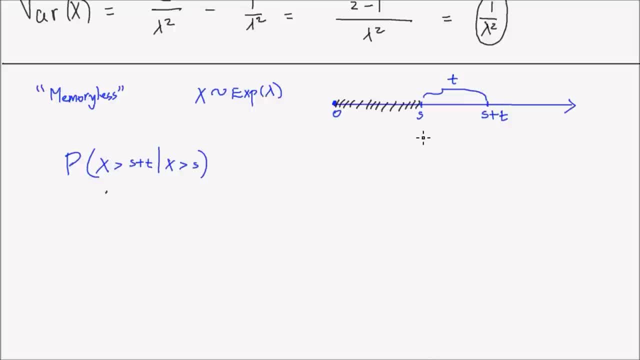 So it does not remember this past. So calculating this probability is the same as calculating the probability that a brand new equipment is going to work for at least t units of time. So what you need to calculate is the probability that a new equipment would work for at least t units of time. 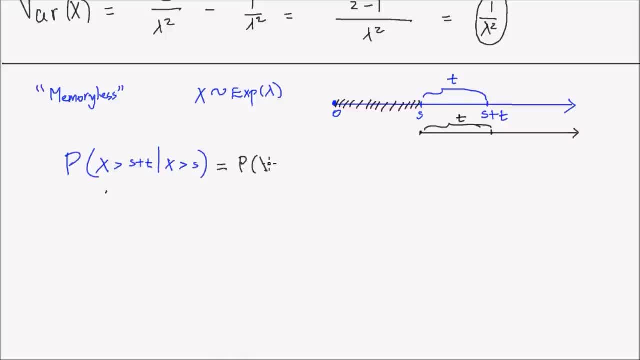 And this probability would be equal to the probability that x is greater than t. So let's see if this property is satisfied for exponential distribution. So let's calculate the probability that x is greater than s plus t, given x is greater than s, This is equal to the probability that x is greater than s plus t and x is greater than s by conditional probability formula.